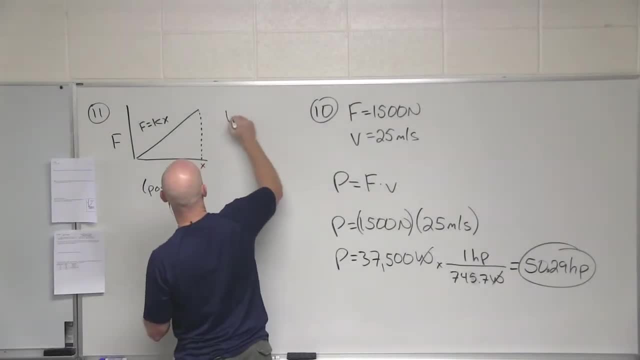 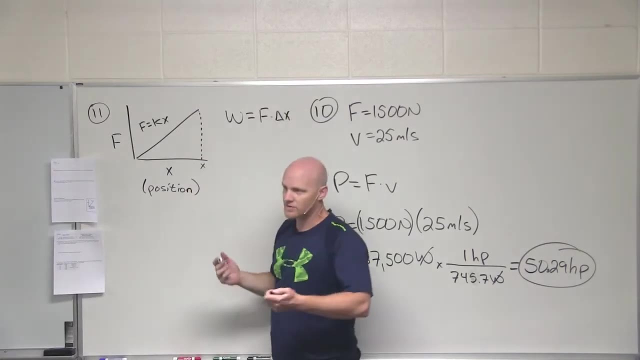 So let's look at your definition of work here real quick again. Work equals force, times, Displacement. I'll call Delta X, or your book calls it D as well. same diff In this case. I like Delta X. In this case there's a definition of work. Now, this definition of work. 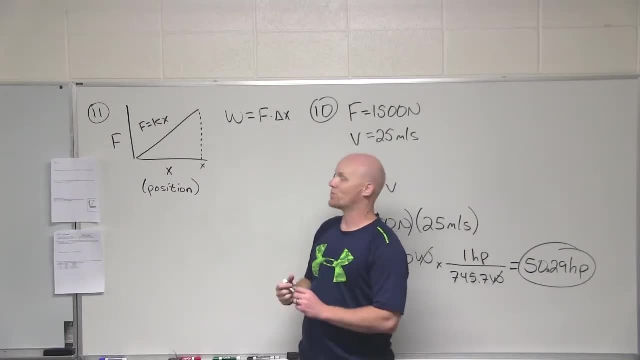 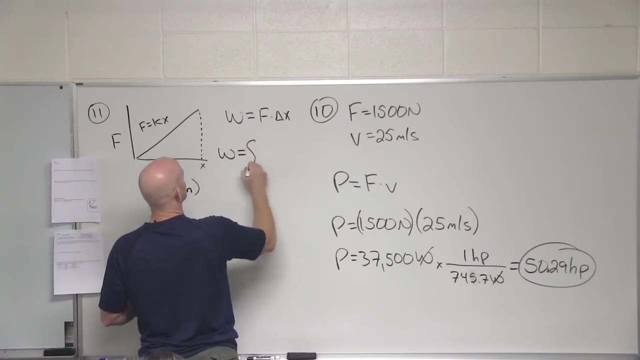 assumes that you've got a constant force, though, Turns out the real definition of work. this is a situational definition of work, but the ultimate definition of work is: work equals the integral of F- DX. How fun is that? You guys like calculus. 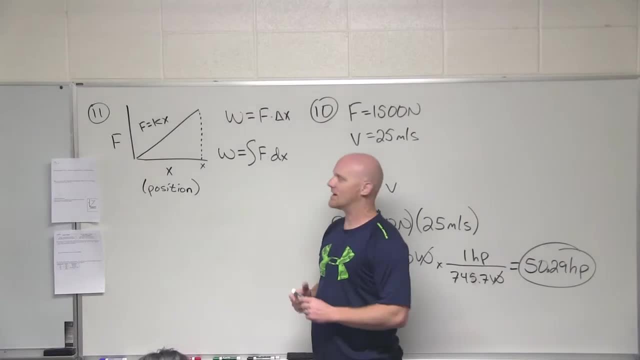 So yeah, so notice, you guys don't need calculus, so. but the idea is this: if your force is constant, if you do know your calculus, you could pull that out in front of the integral. and the integral of DX is just simply Delta X, which is 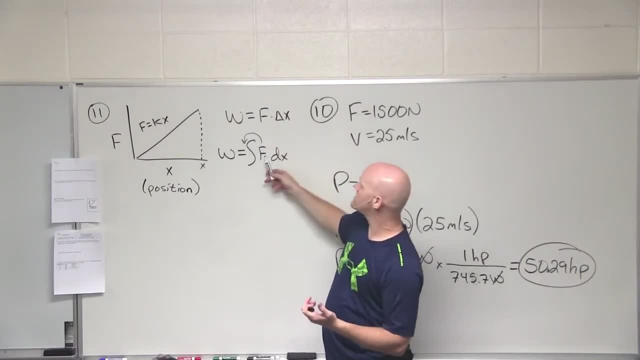 where that comes from: X final minus X initial. So if your force is constant, that's what work turns into. but if your force is not constant, then you can't pull it out in front of the integral And you'd actually have to take a little more complex integral and stuff like. 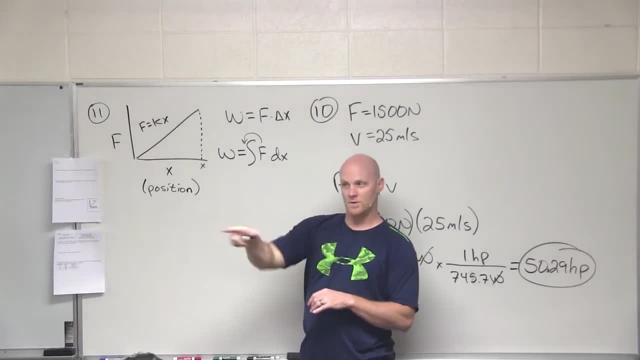 that. Well, if you're a class, you definitely don't have to do that. it's not going to be involved Question: Wasn't there cosine theta? So? so in this case you're right. If F is not in the same direction as the. 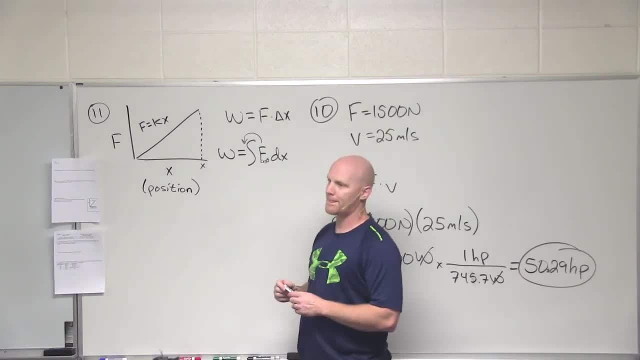 displacement. you've got a cosine theta factored in there as well. So in this section we just take cosine theta out. Well, it's not even just taking cosine theta out. In this case, the question you're going to get is either going to be in the same direction as the 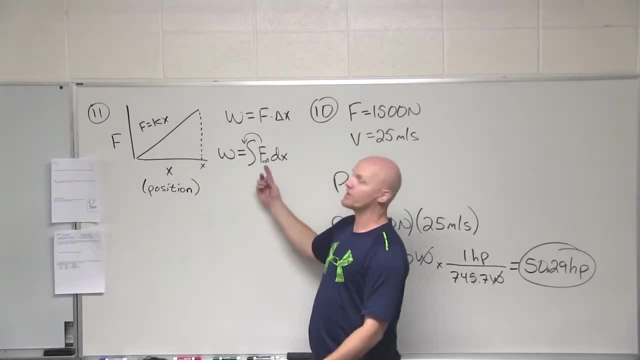 displacement. or you're going to be in the same direction as the displacement, Or it's not. They'll let you know If it's not include the cosine theta. If it is, though, leave it out, because cosine of zero is one, Alright. so in this case, I'm 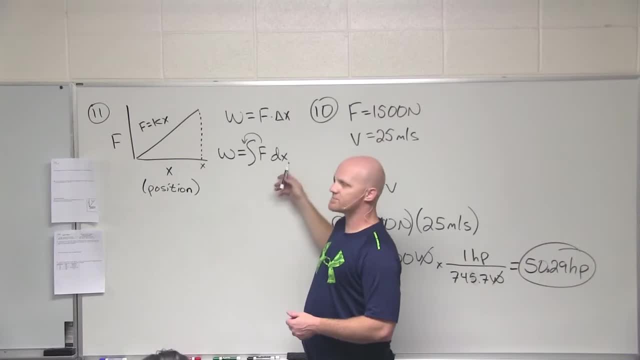 going to leave it out. I'm going to just give you a situation where the force and displacement are in the same direction And in this case, if your force is variable, then we got an integral to take. Have you guys had calculus? Okay, so when? 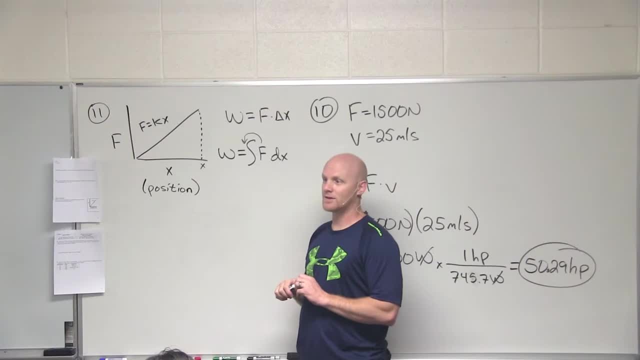 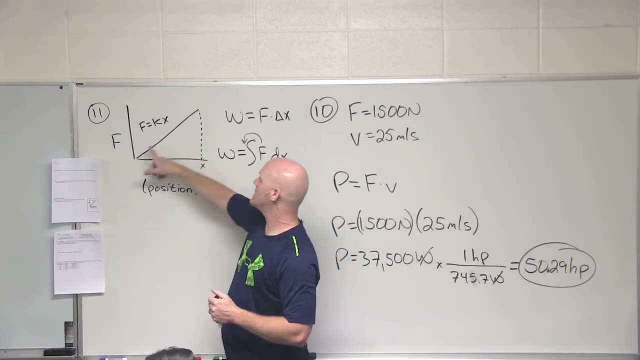 you take the integral of something, that's the same thing as finding or determining Area under the curve. I mean, an integral is an antiderivative but it's finding the area under the curve. So here, if you're given a graph of F versus position, So it turns out taking the integral of F, dx would be the